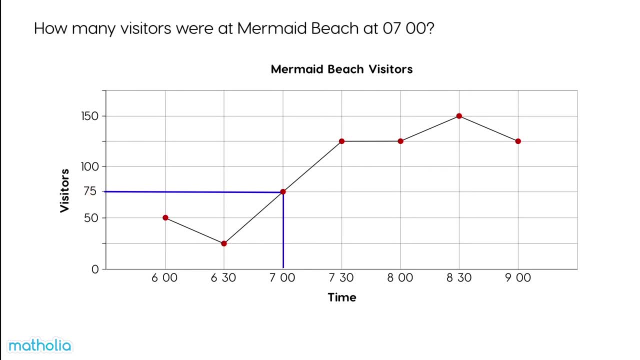 So there were 75 visitors at 7 o'clock. What was the increase in visitors? There was a difference in visitors from 7 o'clock to 7.30.. The number of visitors increased from 75 to 125, which is an increase of 50 visitors. 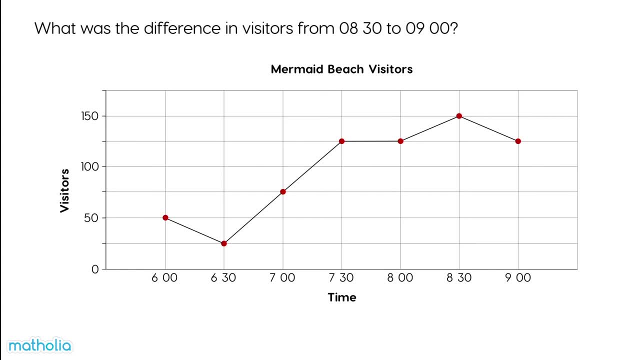 What was the difference in visitors? from 8.30 to 9 o'clock? The number of visitors decreased from 150 to 125. So there was a difference of 25 visitors. So there was a difference in visitors from 8.30 to 9 o'clock. 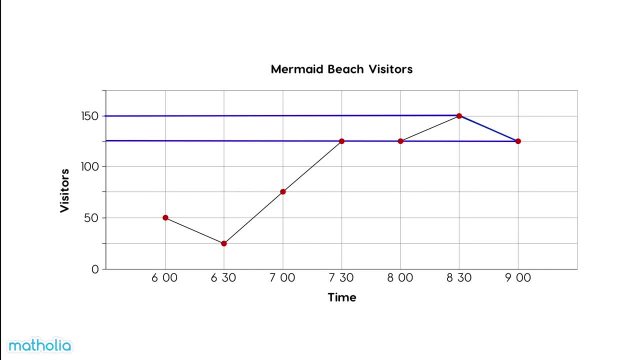 I hope these questions have helped you to learn to interpret line graphs At home. measure the temperature outside every hour for 6 hours. Show how the temperature changes by drawing a line graph. Tell what you can interpret to a friend. See you next time. 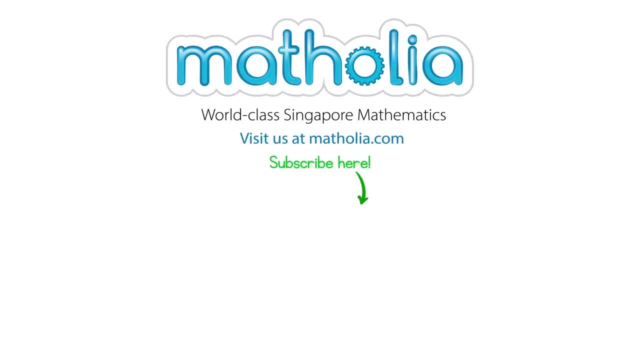